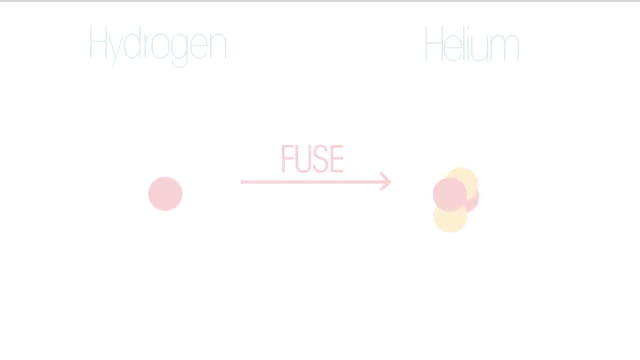 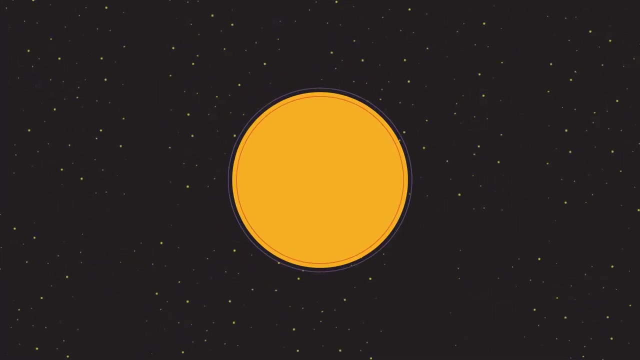 to fuse to form helium. For more about nuclear fusion, watch this video. The star then enters a long, stable period where the outward pressure of the heat generated by nuclear fusion counteracts the force of gravity. The star is now called a main-sequence star and it stays in this state for between 10. 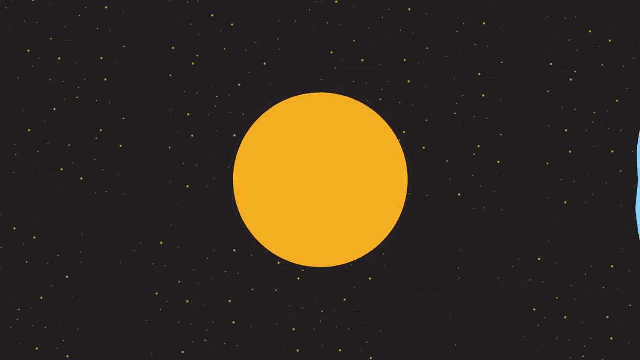 million and 10 billion years. What happens next depends on the size of the star. Let's talk about a smaller star first, one roughly the size of our Sun. Up until now, the nuclear fusion has been occurring between hydrogen nuclei, but eventually. 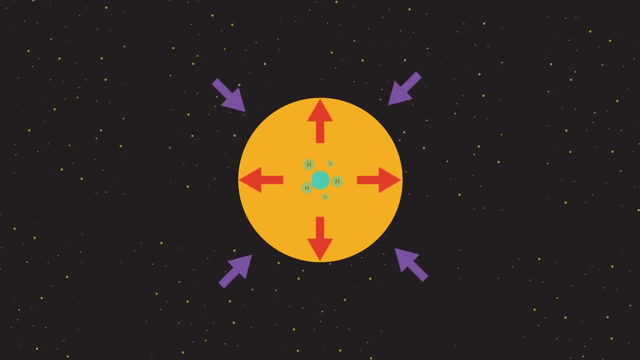 the hydrogen begins to run out. Now the outward force of fusion is less than the inward force of gravity. This causes the star to collapse inward and the temperature to increase. It becomes so hot that helium nuclei can now begin to fuse together to form heavier elements. 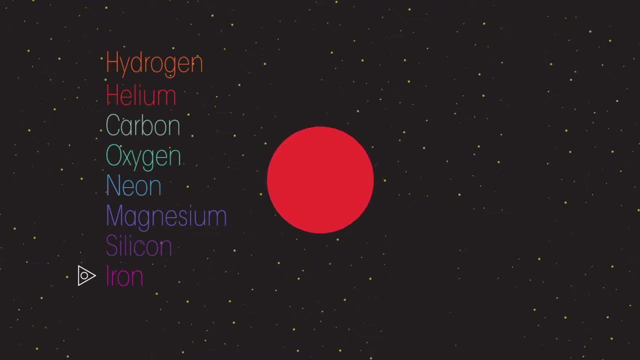 but only as far as iron. To form elements heavier than iron, the star must be heated to the maximum temperature of the star. To form an iron requires an input of energy, which we'll explain a little later. The star now expands and becomes what is called a red giant. 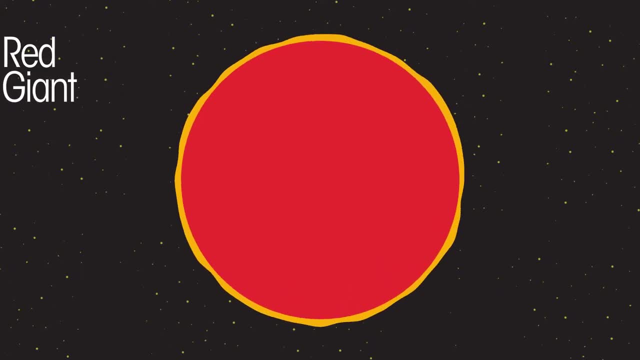 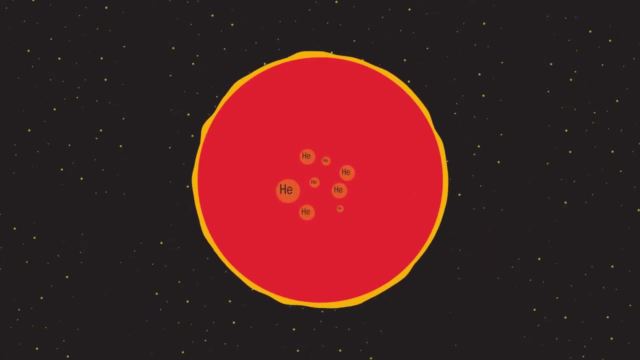 When our Sun becomes a red giant, it will expand to such a size as to engulf the three inner planets. Next, fusion of helium in the red giant will eventually stop. Suddenly, the force of gravity is greater than the outward pressure of fusion causing. 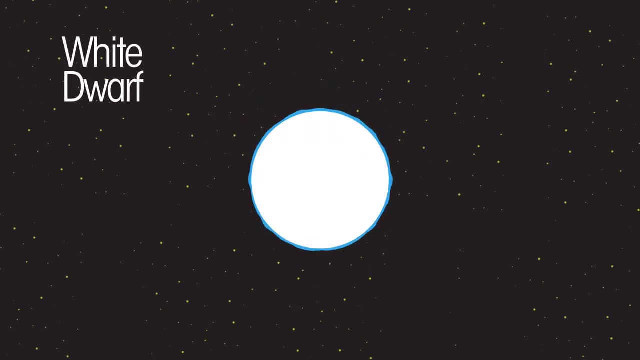 the star to collapse, forming a white dwarf. Eventually, after billions of years of cooling, the black dwarf will stop releasing heat, So no more fusion is occurring inside the star, and so the white dwarf cools down. Eventually, after many billion years of cooling, it stops releasing heat and it becomes a black. 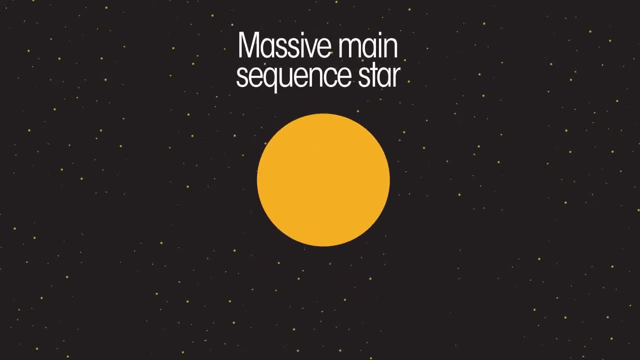 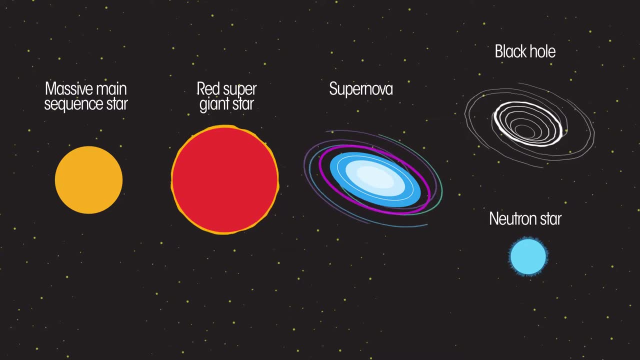 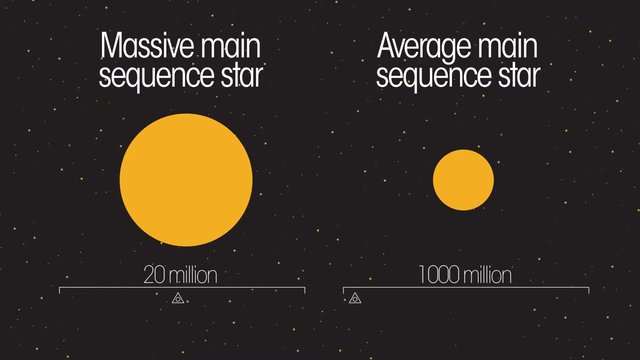 dwarf as cold as the empty space that surrounds it. So what about bigger stars? What happens to them? They follow a different pattern. Stars, too, eventually run out of hydrogen, but quicker than a smaller star would. Massive stars, as a result, have a much shorter main sequence life than smaller stars.